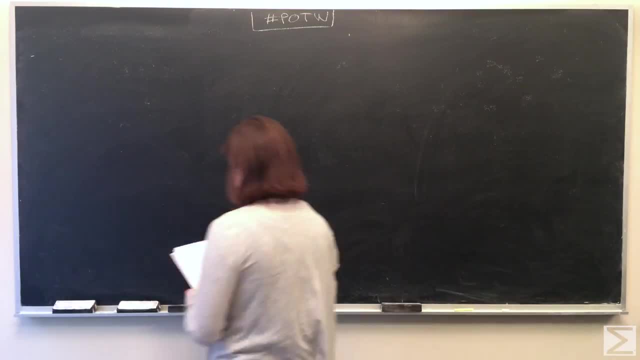 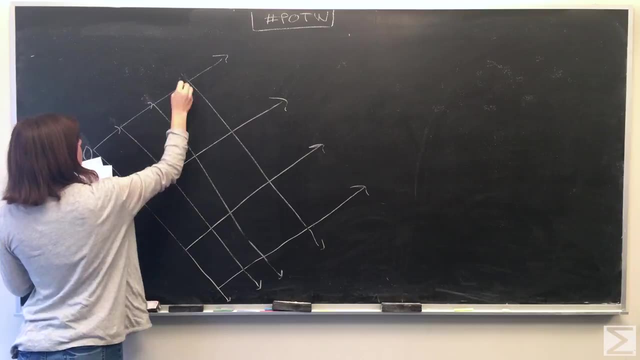 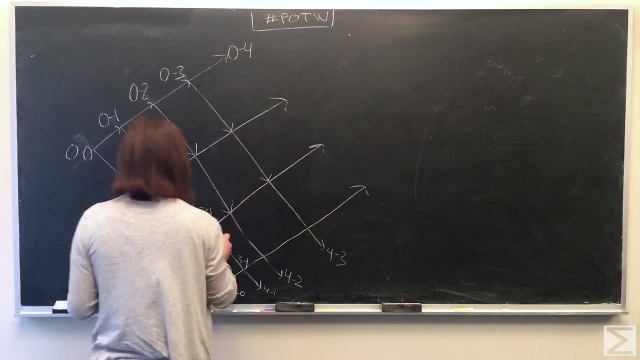 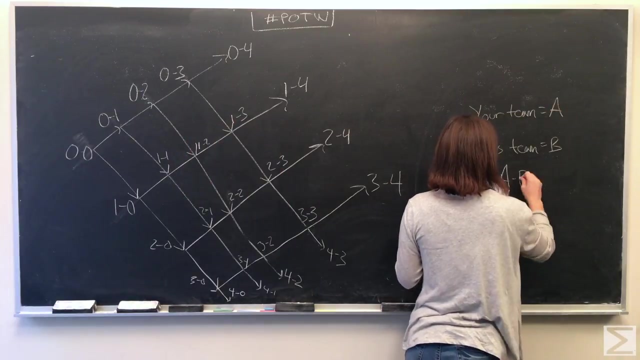 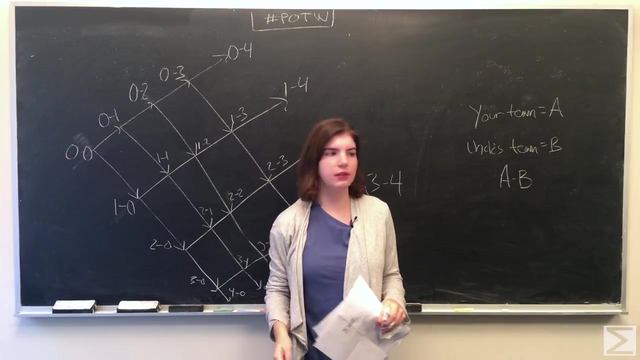 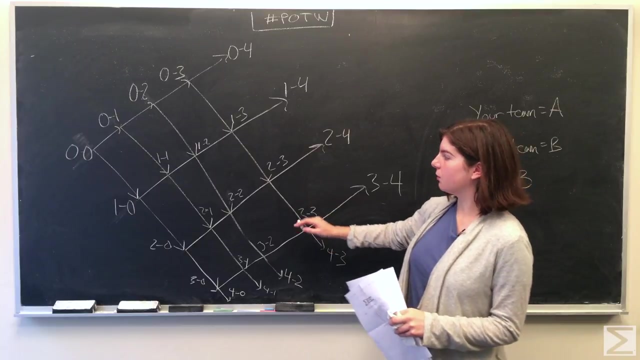 We'll call the team that you want to win Team A. and we'll call the team that you want to win Team A. And the way we have our chart set up is it reads from left to right and if your team wins, it moves down. 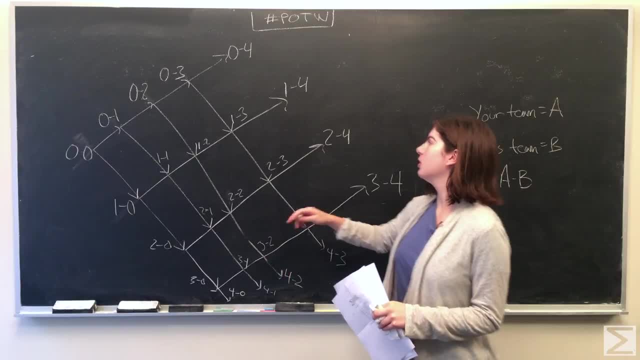 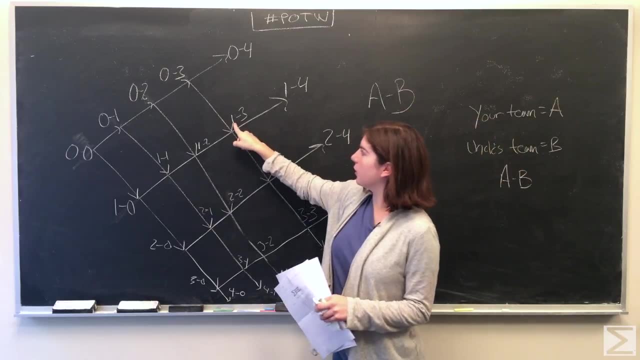 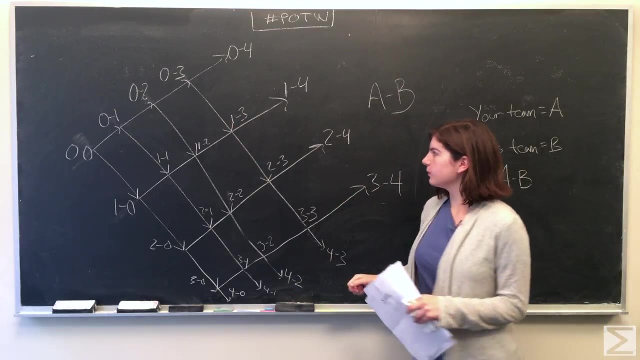 and if your uncle's team wins, it moves up And it reads from A to B score. so if the score is 1 to 3, your team won one game and your uncle's team won three. So we already know that. 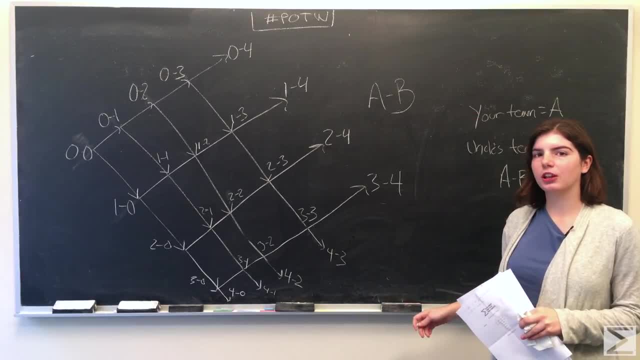 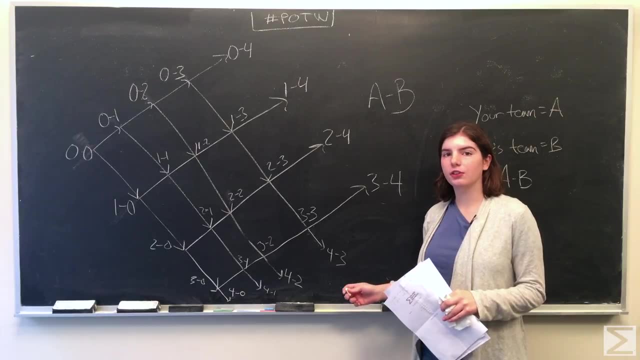 if your uncle's team wins, if we're betting on individual games and they have to win four games to win the series, so you want to walk away with $100 if your team wins the series. Your team wins when the score is 4 to 0,. 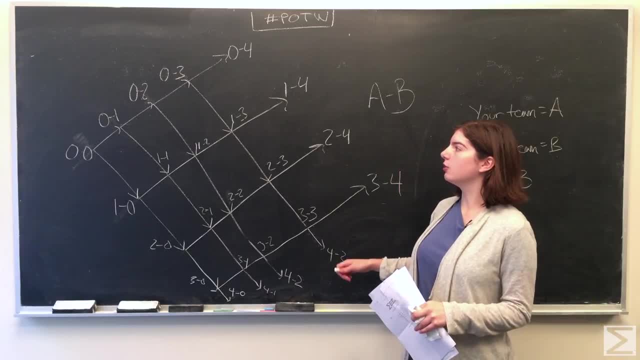 4 to 1,, 4 to 2, or 4 to 3, and you lose if the score is 0 to 4,, 1 to 4,, 2 to 4, or 3 to 4.. 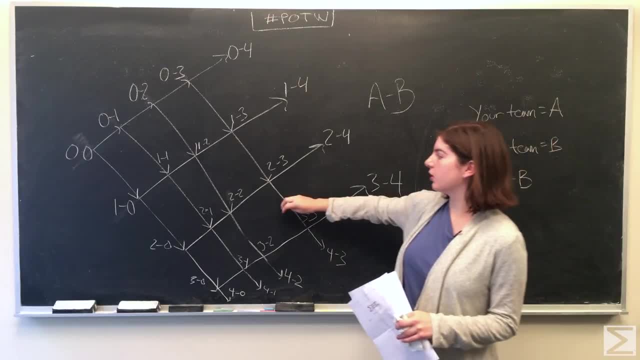 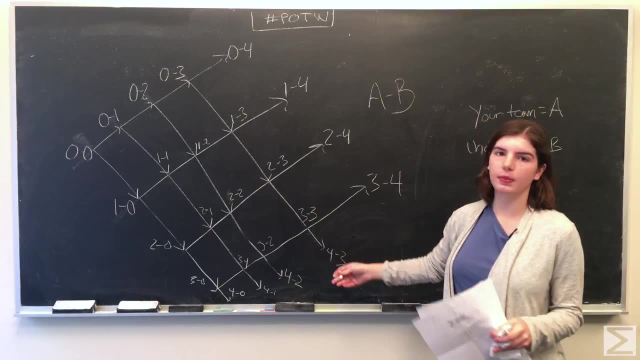 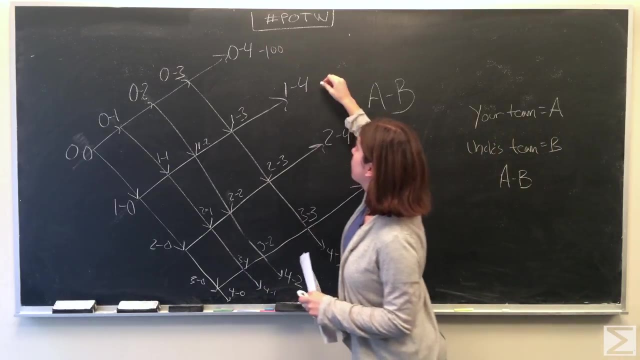 So we can go ahead and we'll write our at each score. you're either going to have a net winning or net losing, depending on how the series is going. So when they lose the series, you'll be out $100.. 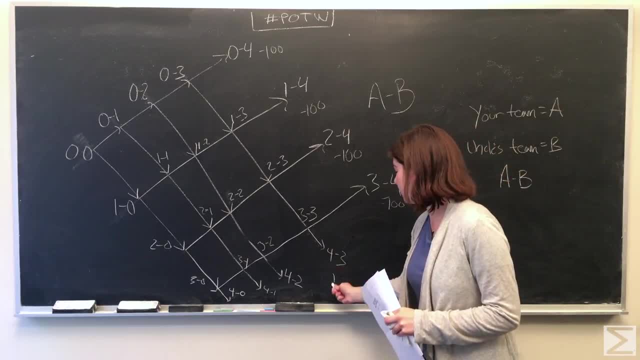 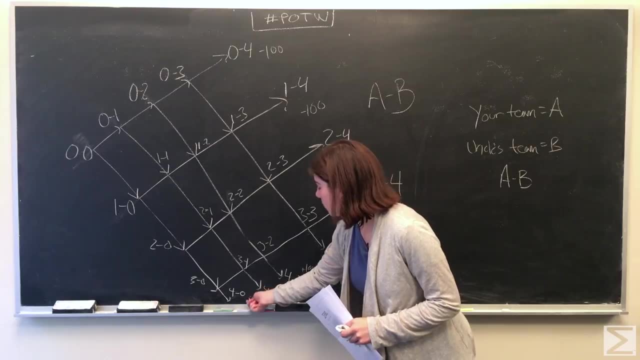 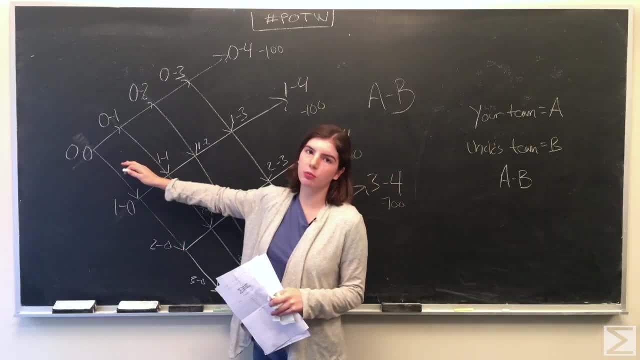 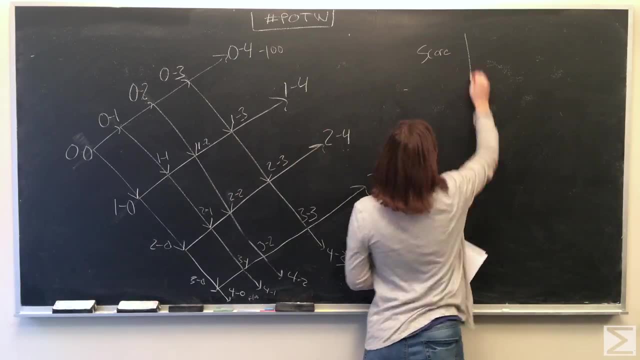 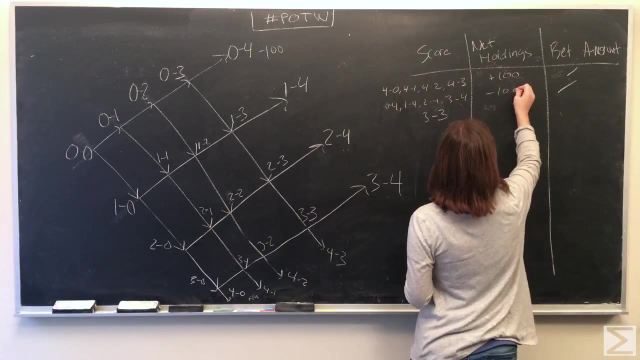 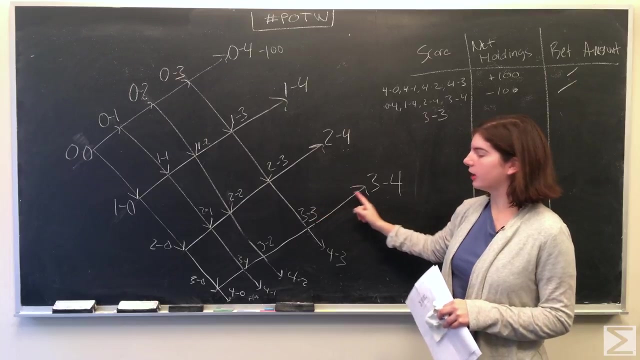 $100. $100. $100. $100.. We're going to work backwards to find out how much you should bet on opening game. We'll make a chart. So when the score is 3 to 3, you have to look at both possible outcomes. 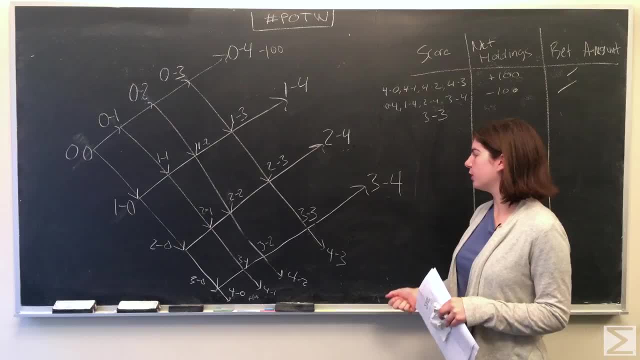 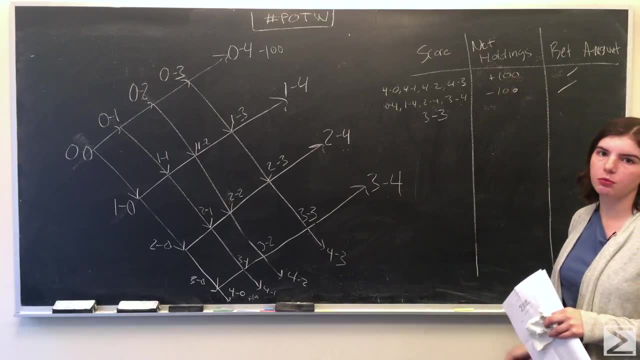 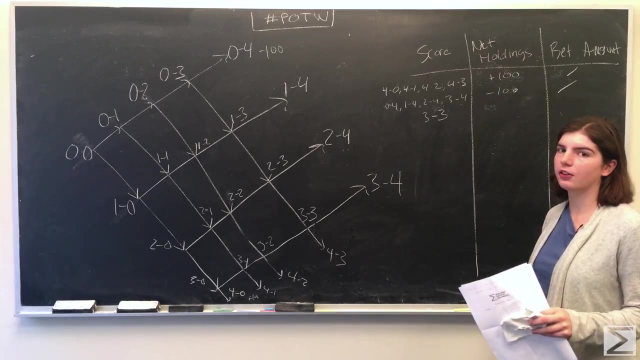 It can either result in the score 3-4 or 4-3.. We know that your net holdings at 4-3 is going to be positive 100 and your net holdings at 3-4 is going to be negative 100.. So to find out your net, 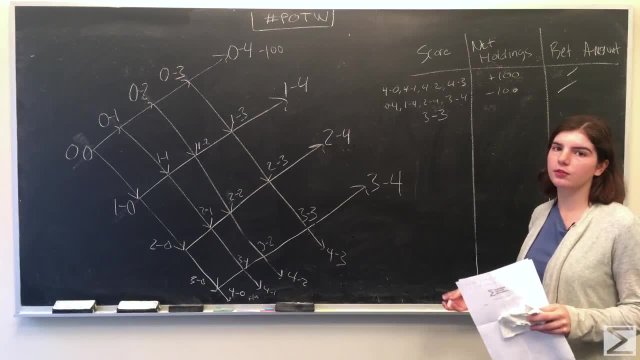 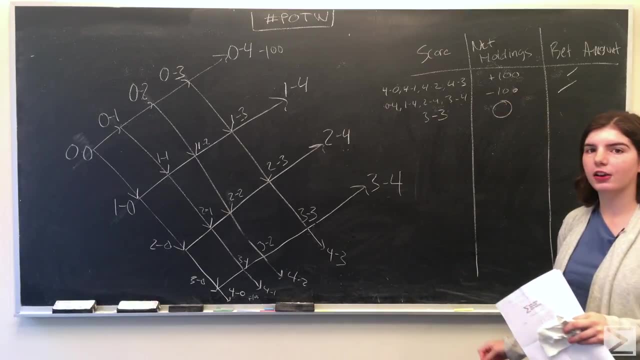 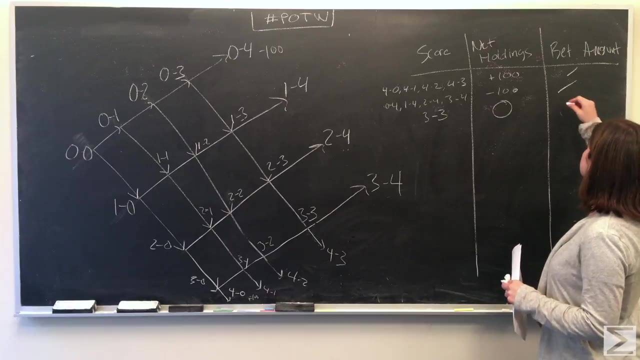 holdings at 3-3, you take the average of the two outcomes, which would be 0. Then to find out how much money you should bet, you're going to take half the difference of the two outcomes and you have to continue on. continue working. 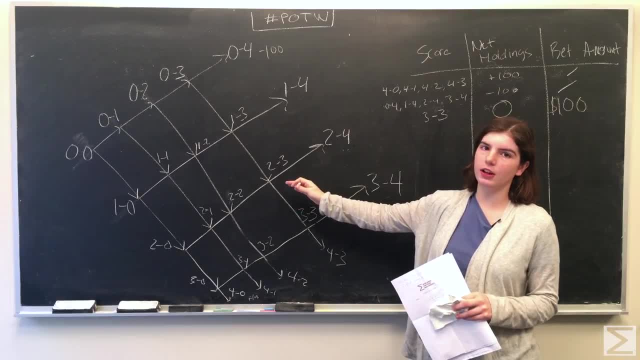 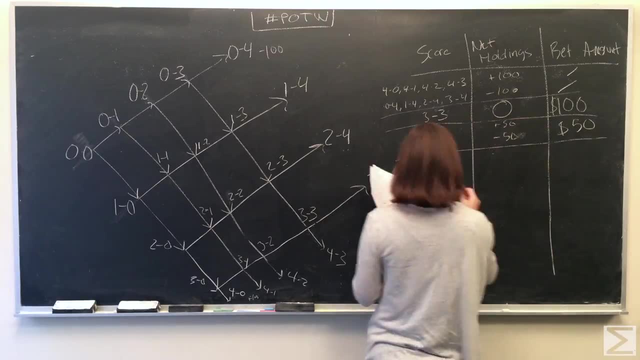 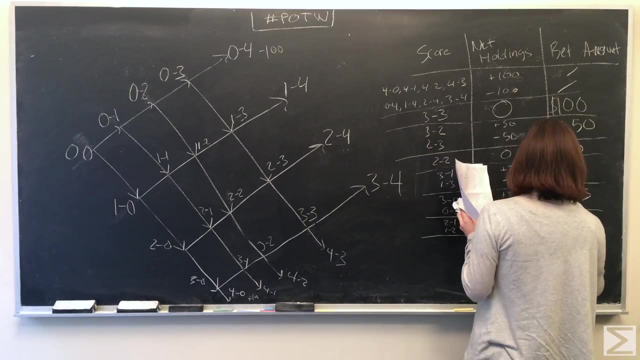 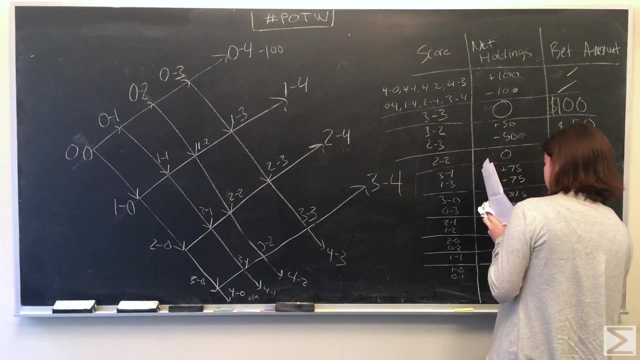 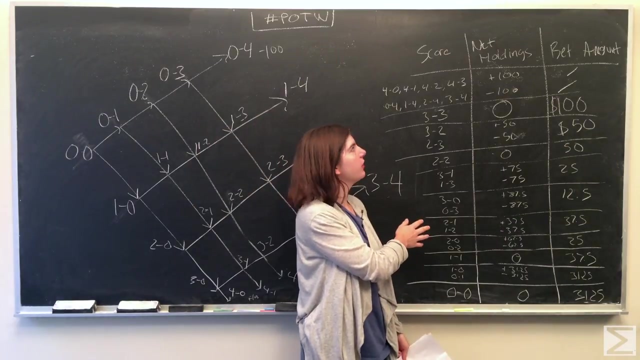 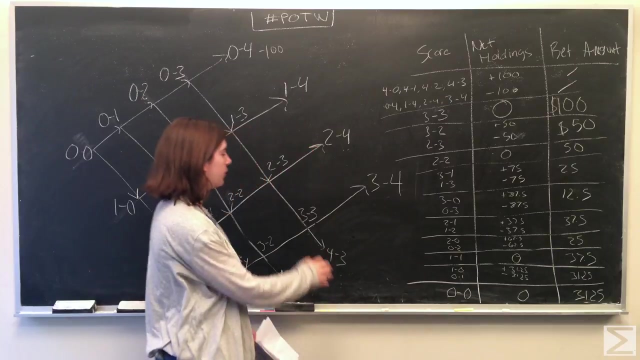 backwards to find out your bet amount and your net holdings at each score. Once again, all we did to find the net holdings was we looked at which game, which score, we wanted to find and we saw it has two arrows pointing to it, because 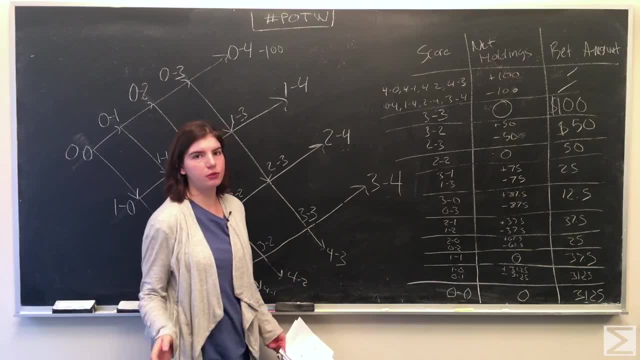 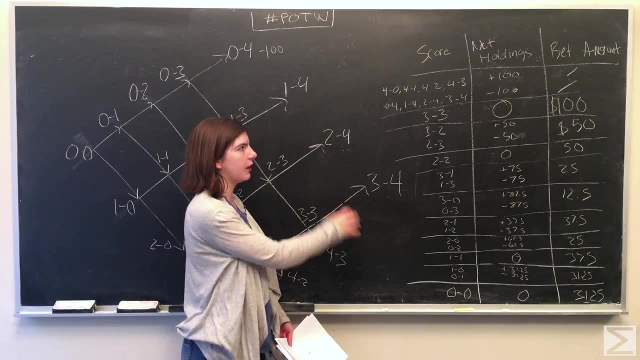 they can either win or lose. Tying is not an option. And then to find out how much money you should bet, you're going to take half the difference of the two outcomes and you have to continue on, continue working backwards. So we knew that the net holdings from the outcomes and we took the average. 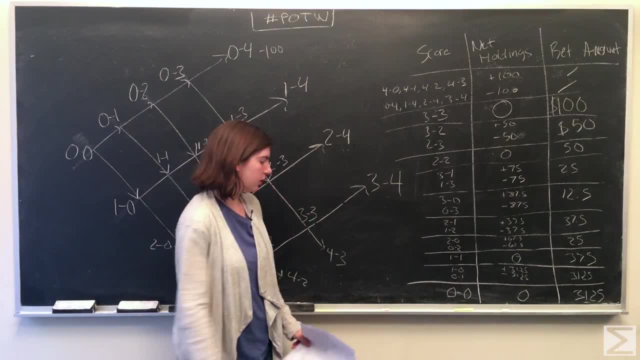 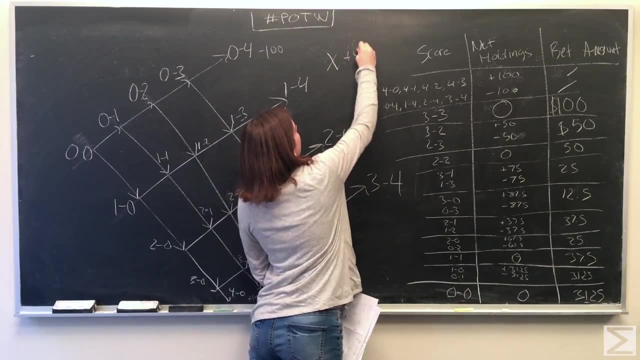 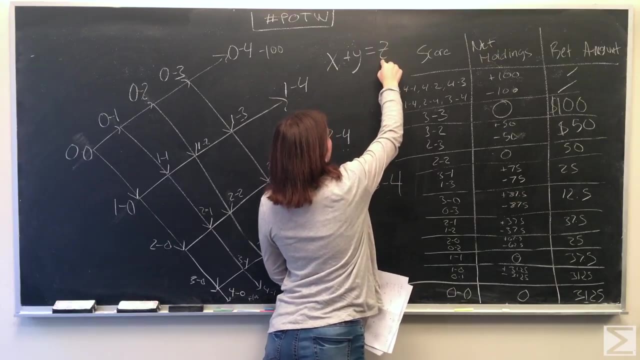 And then, based on our net holdings, you can find the bet amount. because if you take, if X are your net holdings at that game and Y is your bet amount, you know, and Z is your net holdings at the next outcome. so then your bet amount. 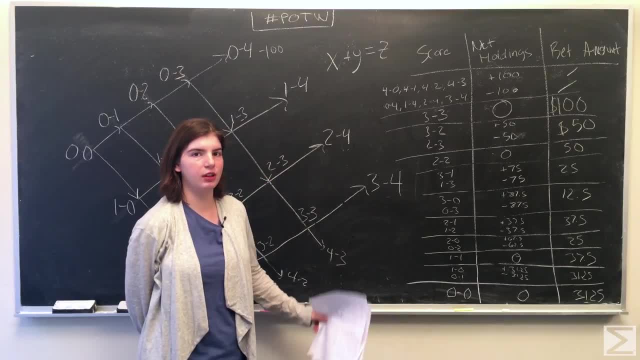 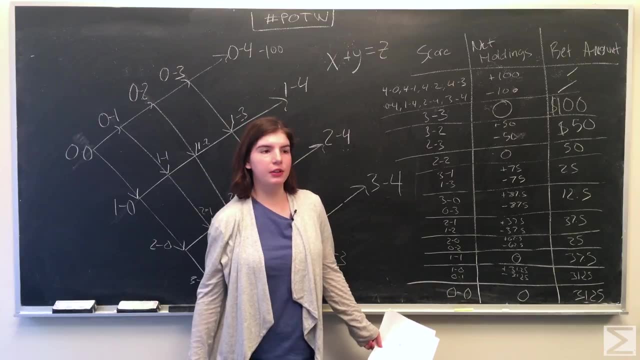 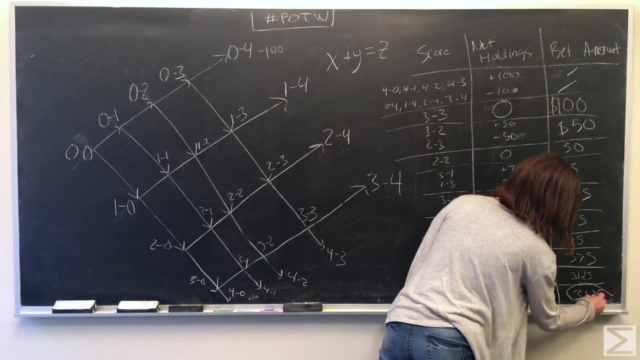 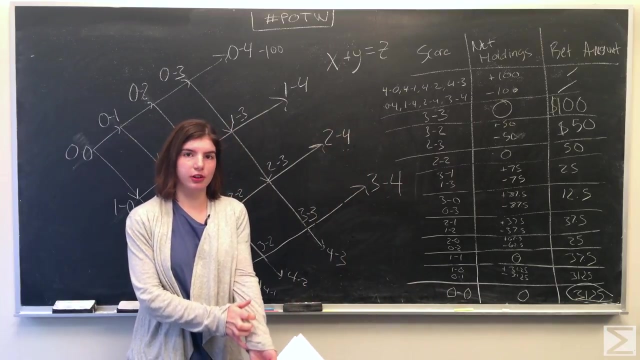 would be half the difference of the outcomes, And once you work your way down, you see that the bet amount at the opening game should be $31.25.. Thank you for watching. I hope you enjoyed this video. Be sure to comment below which teams you want to see make it into the World Series and check. out our blog And follow us on Twitter and Facebook, Thank you.